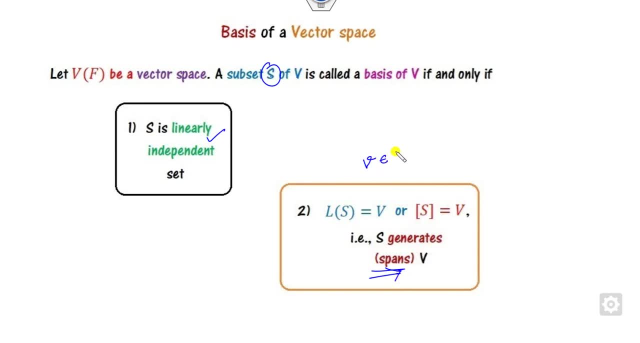 is the span of that. It means if you take any element of from the v, then it must be written in the form of a vector space. So if you take any element of from the v, then it must be written in terms of the elements of the s. Every element of v is written as a linear combinations of the. 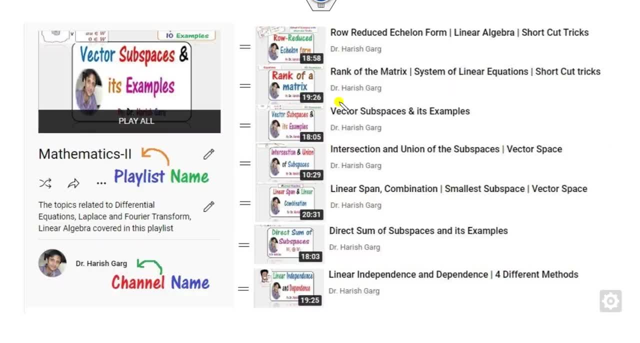 elements of s. So we already discussed these two lectures in my last, that is, you can see the linear span combinations and the linear independence lectures are there. where you can see the various methods in order to solve such problems are there. So all are available in the channel name. 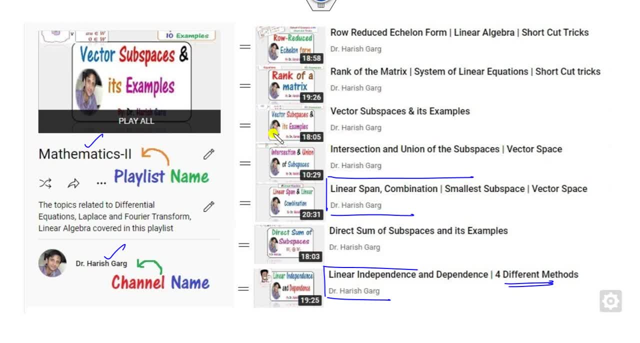 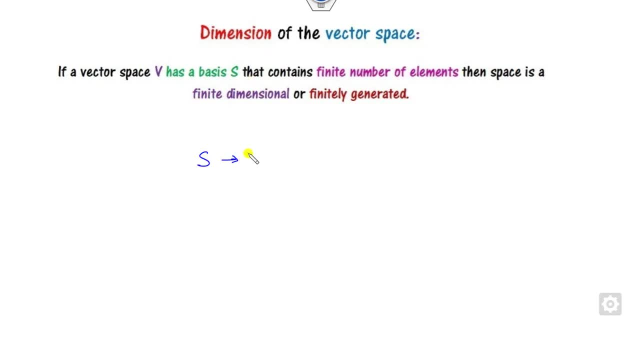 Dr Harishkar. Mathematics 2 is the playlist, So you must watch these two lectures before understanding this today's lecture. S is my basis. then my question arises is how you can find the dimensions. So if you have proved that s is a basis, it means it satisfies the two properties. one is the linear, independent and 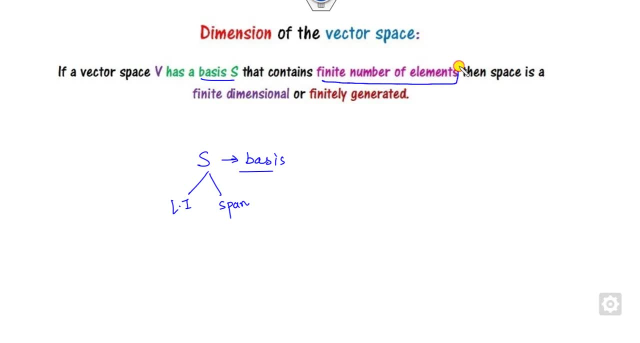 second is the span. then how many elements are involved in this? in this s, If it consists of the finite number of the element, then we call as the finite dimensions, and the number of the elements of this s is called as the dimension of the vector space. It is denoted as d i, m. 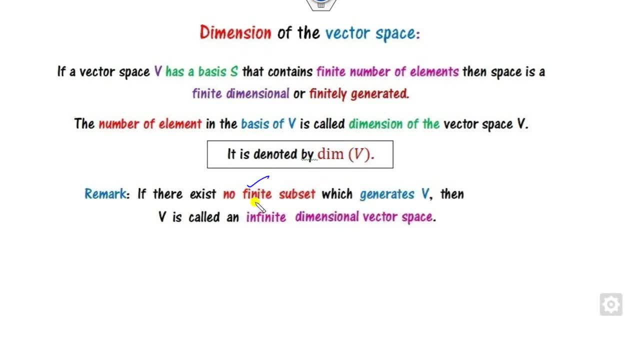 of v. If you are unable to find any of the finite subset, then it is called as the infinite dimension space, For example. so assume that this is my basis. so firstly, you have to prove that it is a alliant span. it is clearly seen that it is a alliant span. Now what is the dimension of the v? 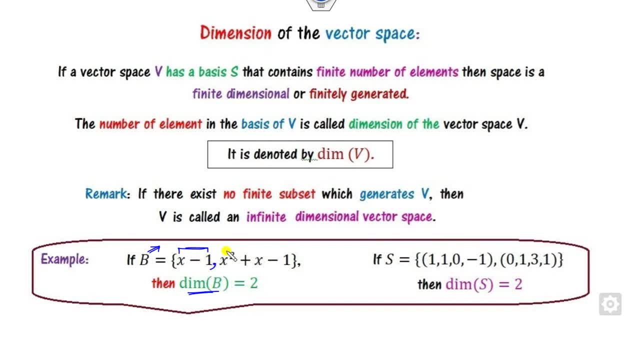 how many elements are there. you can see: this is the first element. this is a comma. this is the first element. this is the second polynomial, so there are the two polynomials. so that's why i say: dimension is two. This is a one vector. this is the second vector. so that's why dimension is my two. 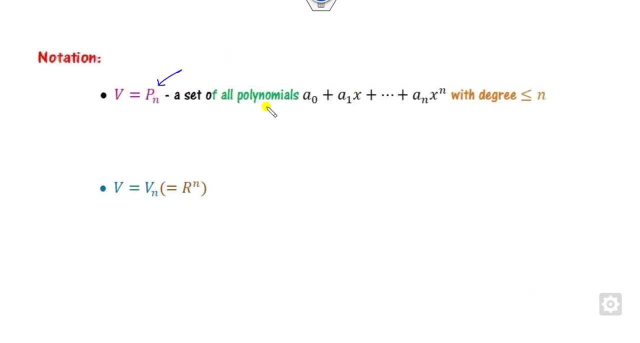 We will denote it. p of n is a set of all those polynomials of degree less than equal to n, like here, and v of n is a n dimensional vector space, like what is the v2? v2 is nothing but my r2, that is a xy plane. what is our v3? v3 represent for my r cube? that is a x, y, z plane. r and this is my. 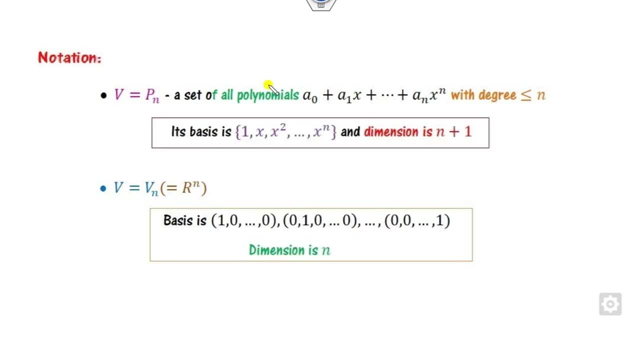 xy here Now, once you are here, then, what are the basis of this? what is the coefficient of the a0? is the symbol by 1.. x and x raise power n. how many elements are there? this is n plus 1.. What is the basis of this? is the 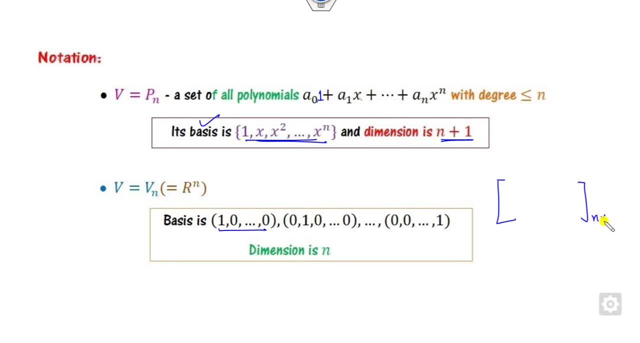 first, this is the identity matrix. what is the i matrix of the n cross n? this is 1, 0, 0, 0, 1 and so on. and this is 0 0, 1 is there, and dimension is my n. Remember that whenever there is a polynomial, 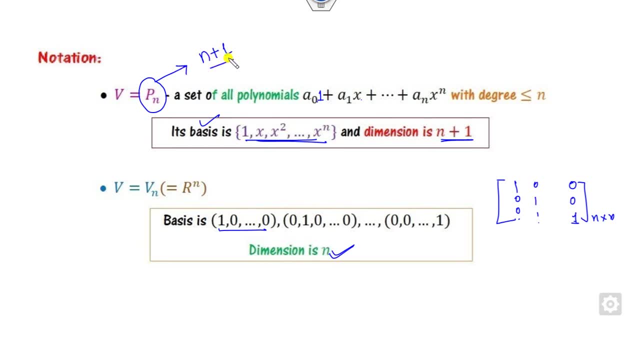 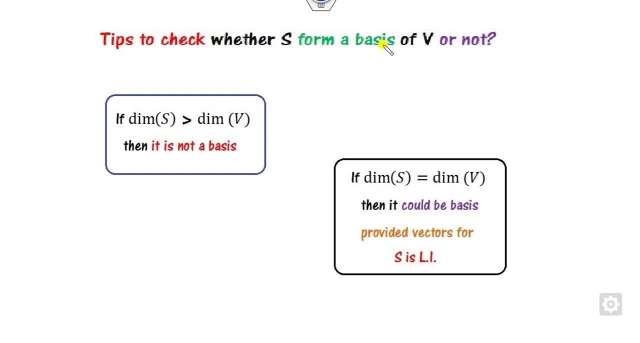 of the p, and that dimension is my n plus 1.. How you can prove that, whether the basis s is a is a basis or not, you have. i just simply tell you a shortcut: If you have find that the dimension of the s is greater than of the v, then it is not a basis. why? 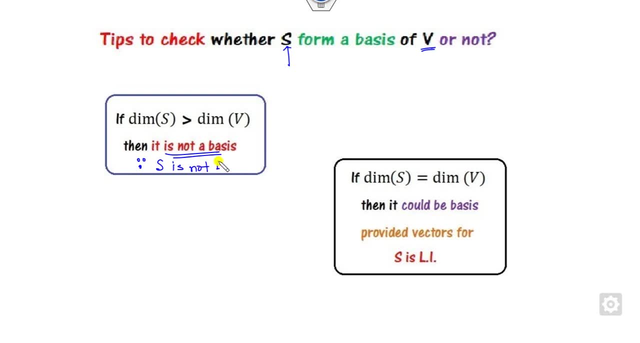 because in that case s is not li. we already discussed in the li lecture what will happen if number of the elements in the r like, say, if i consist of the, this one, vector 2 and the three vectors over the r2. now what is the dimension of the r2? is my 2, how many elements are there? 3? so 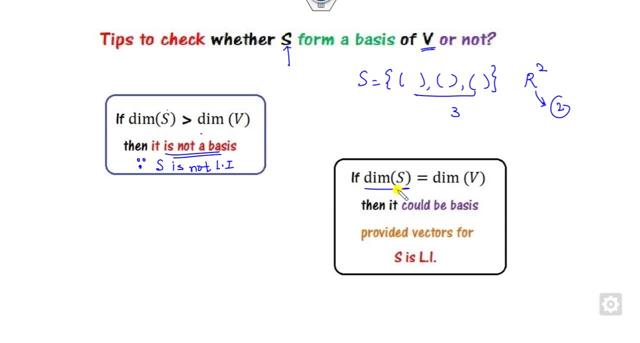 it is not a li, so it means this is not a basis. Prove that it is a less than it is a. if it is equality, then it could be the basis, provided you just simply prove s is li. only there is no need to prove that s is a span. however, if you are able, 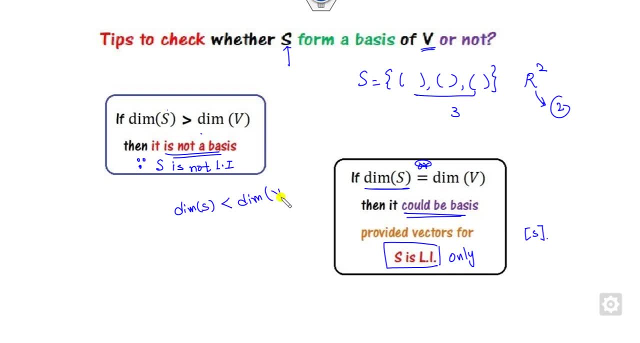 given that dimension of the s is greater than of the v, then you have to prove the. both the things are: s is li and the span of the s is my v. So remember these beautiful tips for you to get the shortcut one, For example here. so what is the dimension of this n? cross n. cross n is a basis. 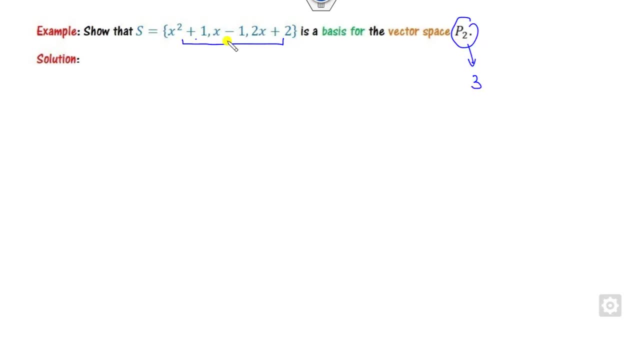 p2, 3. what is the dimension of this is 1, 2 and 3, so since both are equal, so it means there is enough to prove that it is a basis when s is li. if it is not li, then it is not a basis. How you can. 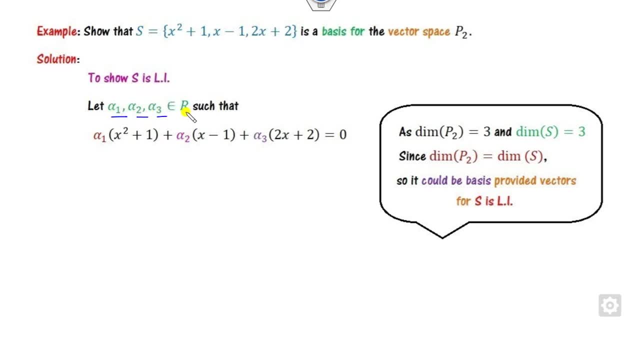 prove that it is a base li. so you can consider the three alpha scalars such that here then your target is to prove alpha 1, alpha 2 and alpha 3 are 0. if they are 0, then we can say it is a li. 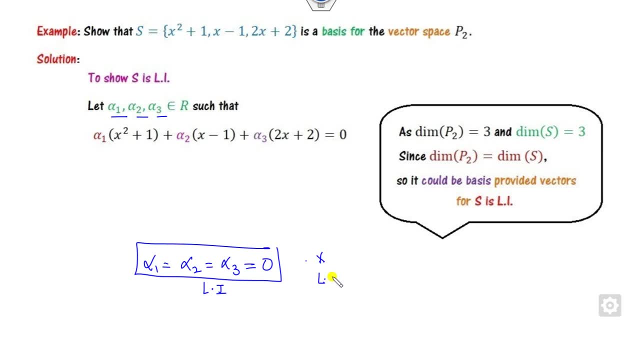 if at least one of them is a non-zero, then we call as the ad. now how you can equate? you can equate the coefficients of the polynomial x. here x and the constant are there. now from here you can clearly see, is alpha 1 is 0. if you substitute here you 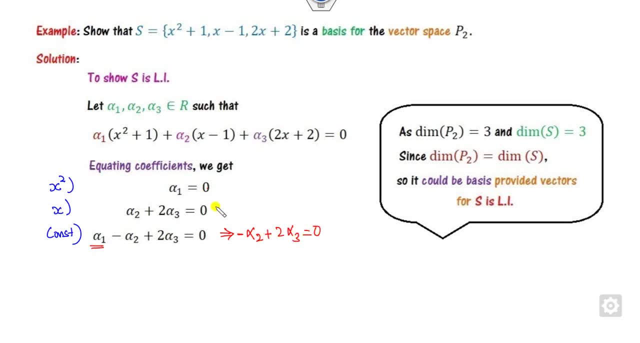 will get minus alpha 2, plus 2. alpha 3 is 0 and from here you will get this value. now, if you add them, what will happen? if you add them, you will get 4, alpha 3 is 0. it means alpha 3 is 0 once alpha 3. 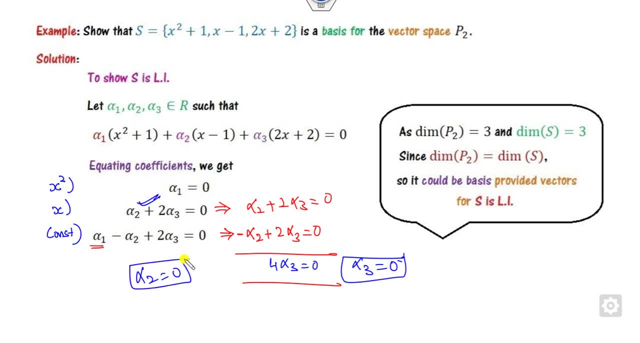 you can substitute here you will get. alpha 2 is also 0. therefore alpha 2 is 0, alpha 1: 0, alpha 3: 0. it means this is li and then, yes, it is a basis. now we can see how you can solve the type 1, where some 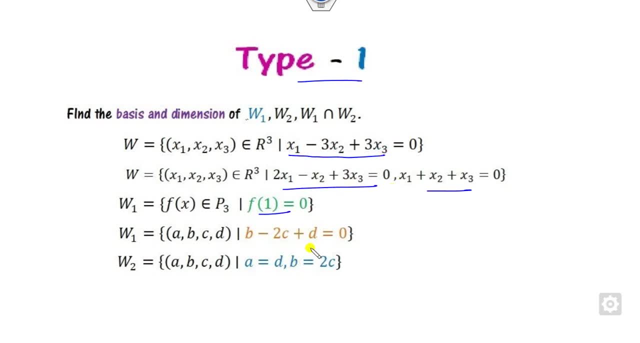 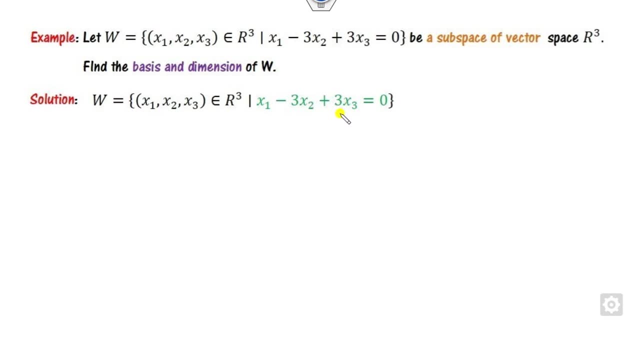 condition is imposed on the problem. so let us discuss all these problems are here, find the basis and the dimension of this. that trick is very simple. what you can do is from this: whatever the relation is given to you, you can solve the problem. so you can solve the problem. so you can solve the. 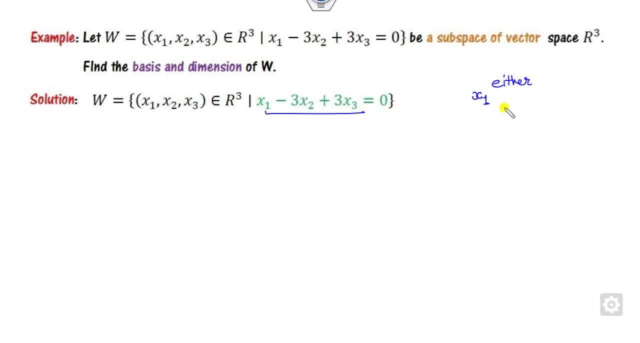 bullshit. in this way i can help you solve this. but before that, what you need to also think about is: what is the relationship between this 2 and this? 2 is 0? you cannot just find the difference here. you only find the organization is coming. you have to find any opposite you can maybe find. 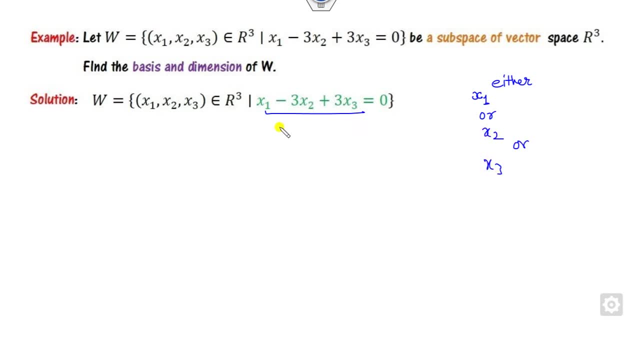 any relative value of this. this say x 1 or x 2 or x 3. you can find either x 1 or x 2 or x 3. you can find. any. of the values are there. now i can find the value of the x 1 because it is quite easy. 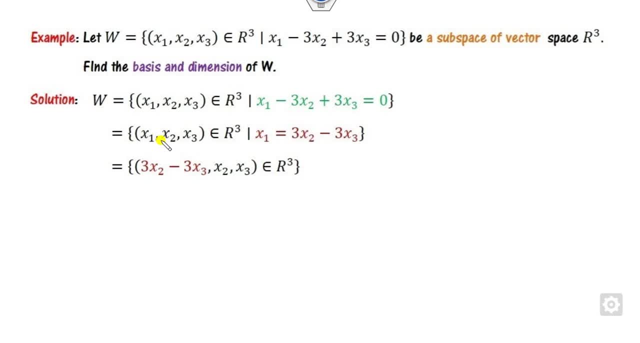 now i can substitute this value of the x 1 as here you will get this expression. now you can see all the expressions are written in the form of the x 2 and x 3. now you can equate the coefficients in the first part. what is the coefficient of the x 3, x 2? there is a 3 comma. what is the coefficient? 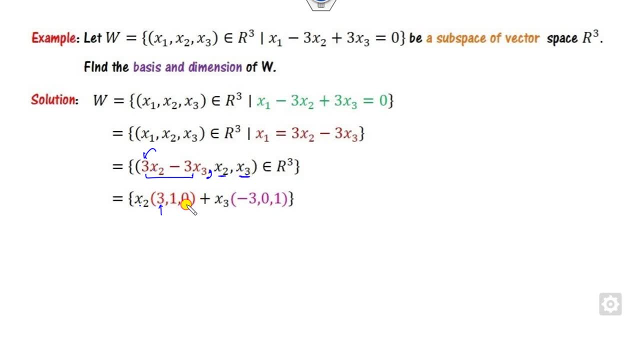 of the x 2 is there one? what is the coefficient of the x 3 that is equal to this here and this is of the x2 here that is nothing is 0, same for the x. now, these two elements are are my basis, and this x2 and x3 are called as the independent vectors or independent elements are there. so the 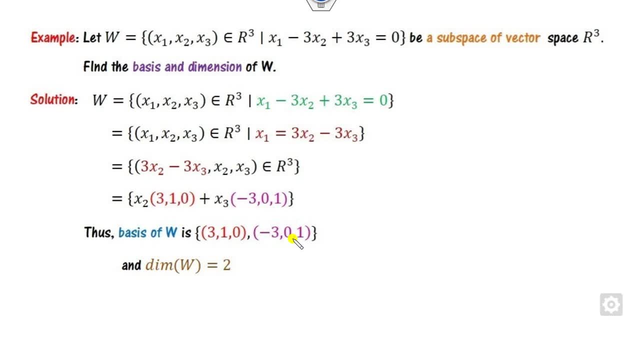 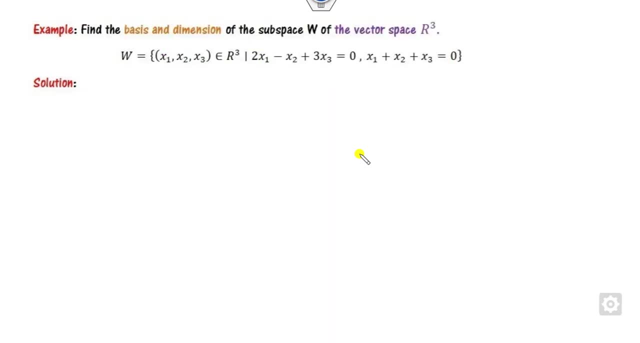 basis are my. here now you can find the dimensions. dimension is my 2, so this is the way you can solve such kind of the problem in a very simple two or three steps are there? look at the one more example. so again, this condition is given to you. now you have to solve the two problems simultaneously. 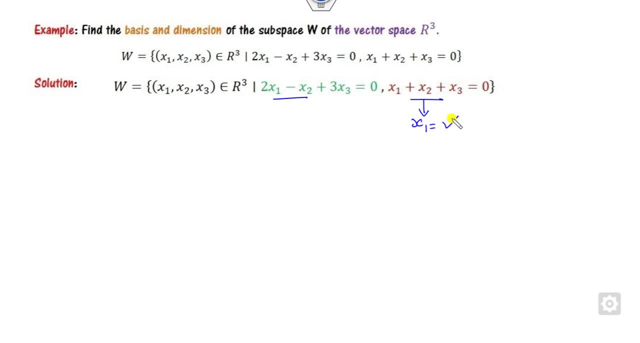 so from here can you find the value of the x1? you can easily find the value of the x1 instead of substituting this x1 here. firstly, we have to solve these two problems. i can substitute the value of the x1 here. you will get this expression. now you can simplify this. these values. after a simplification. 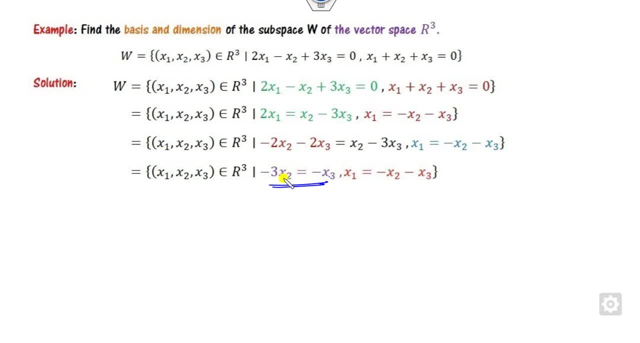 you will get this one now. this is the x3 in terms of the x2. so our target is right here. i can substitute the value of the x1 here. so i can substitute the value of the x1 here. so i can substitute this x3 here. you will get this now. you can see, i can express the x1 in terms of the x2. 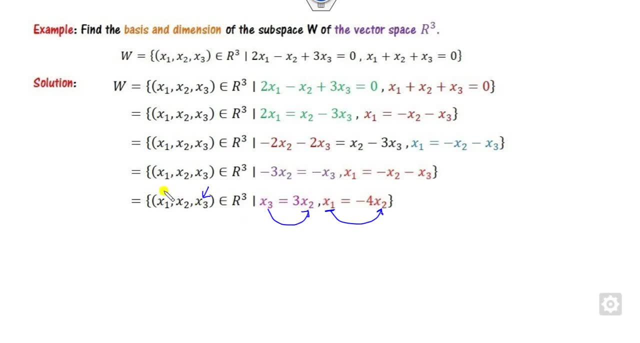 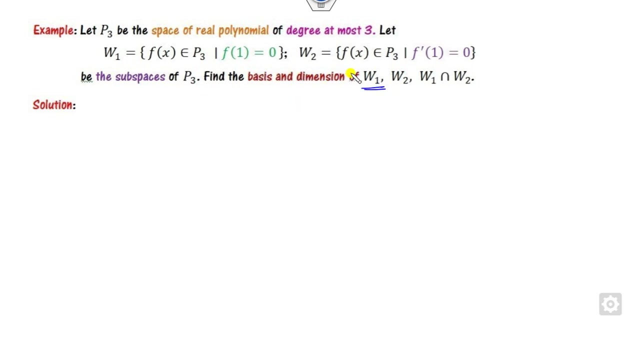 x3 in terms of the x2. now i can substitute both the values at here. you will see this expression. now x2 can be common, so there is only one element. so the dimension is my one and the basis is only w. look at the another one is there where your target is to find the basis and dimension of w1. 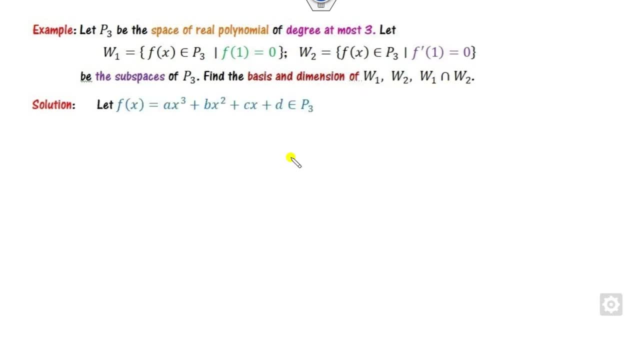 w2 as well as their intersection. so, since it is a polynomial of degree, at the most three. so firstly we can write like here: so let's start with the w1. can you find the value of the f1 from here? yes, you can easily find this. 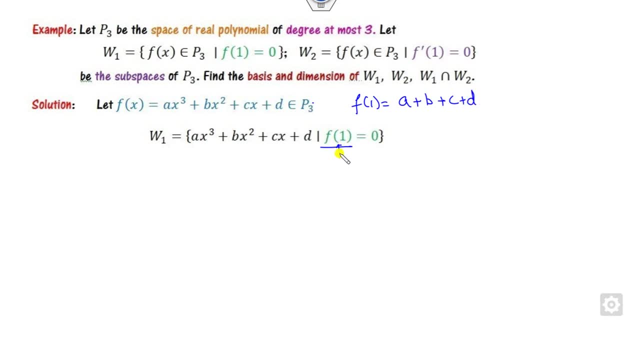 is a plus b plus c plus d, so i can substitute the value as here. now again you can find either as a value of the a or b, or c or d, that's depending upon you. so i can find the value of the a. i can substitute the value of a, as here. you can write this way: now all the expressions. 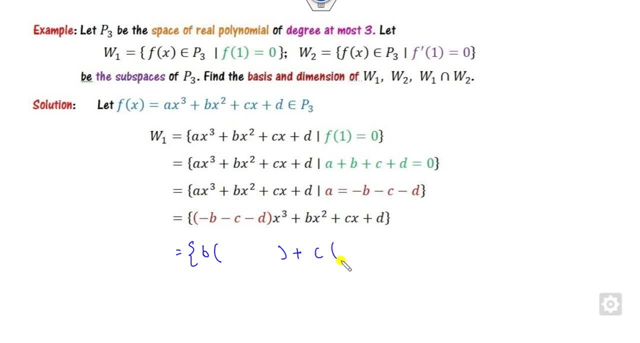 written the terms of the b, c, d so i can take the coefficients of the b, c and d, r so you can see what is the coefficient of the b, my x, cube and so on. so these are my bases and the independent vectors are my three. so b, c, d are my independents and these are my bases, similarly for the w2. so 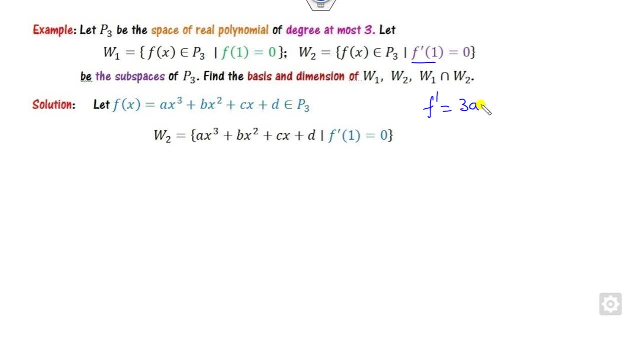 your target is to find the f dash. what is the f dash is there? this is a 3x square plus 2bx plus of c. can you find f dash of 1? yes, this is 3a plus 2b plus of c, so i can substitute here. so from here. 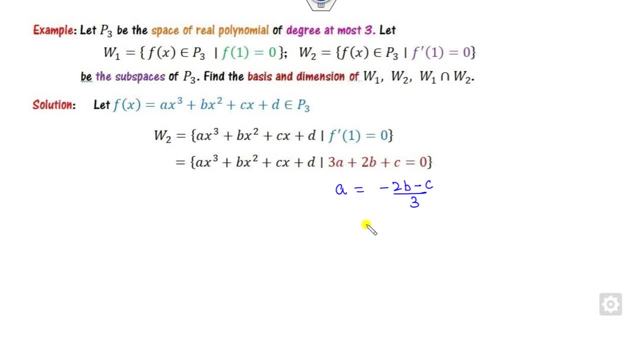 can you find the value of the b a? this is my this- or you can find the value of the b, that's upon your choice, or you can find the value of the c, that's on your choice now, since c is quite easier calculation as apart from the fraction. so i can find the value of c, substitute the value of the. 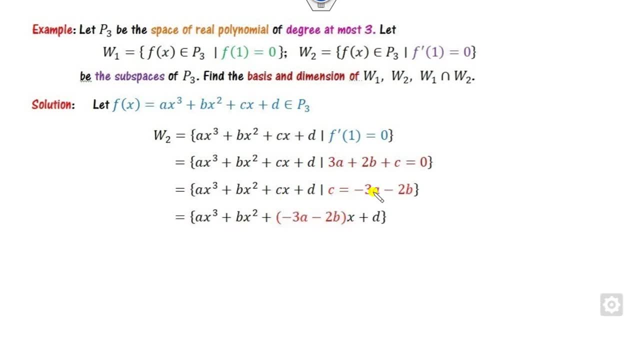 c. here you will get this. now. equate the coefficients in terms of the a and b. you will get this as my basis. now you can see, the coefficient of the d is my 1, so it's it's a 1 scale. similarly, how you can find the intersection, what is the meaning of the intersection is, and so i can write. 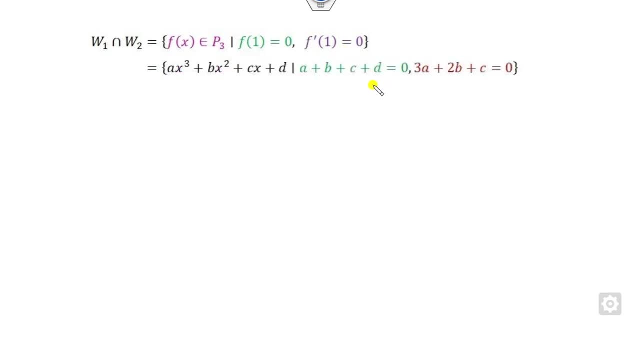 these two pairs, as now i can take these values now. firstly, we have to solve these two problems simultaneously. we can find the value of the c from here and substitute the value c in here, so i can substitute the value of c here. now i can write the c in terms of the ab, so i can solve them. 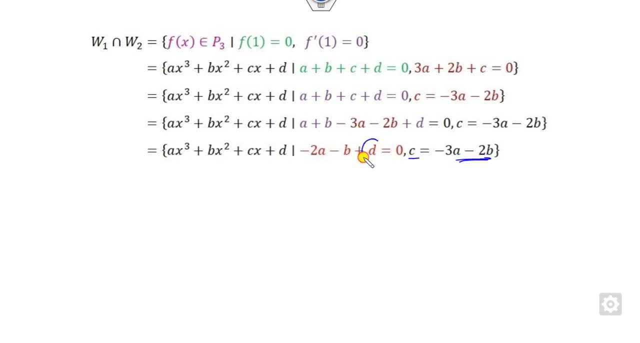 and here c in terms of the ab. so i can express the d also in terms of the ab, as here. now you can see i can substitute the c and d here. you will get this. now all the expressions are written in terms of the a and b, so your target is to write like here. so you can see there are the two elements. 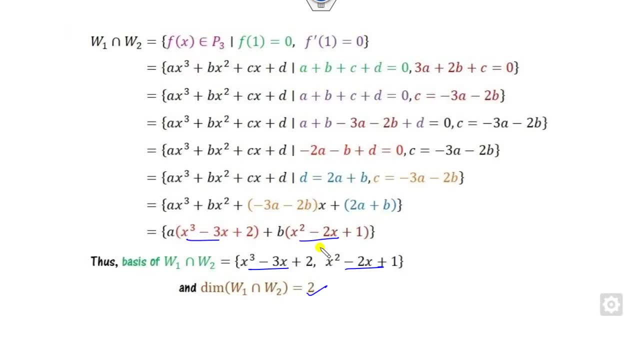 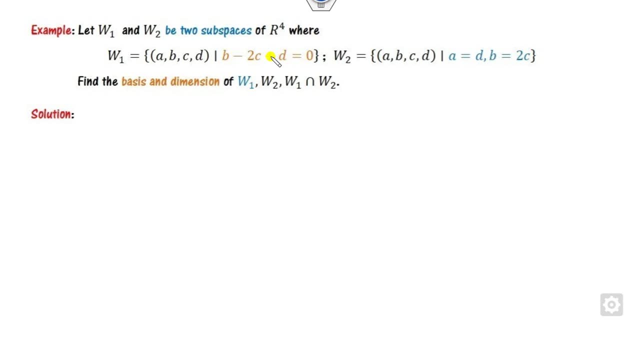 so the basis are like two and the dimension is also the same. so you can see that the basis is my 2. look at the another r there. so again you have to write the w1, w2 and their intersection. so again from here you can find the value of the b or c or d, that's depending upon you. so since b, 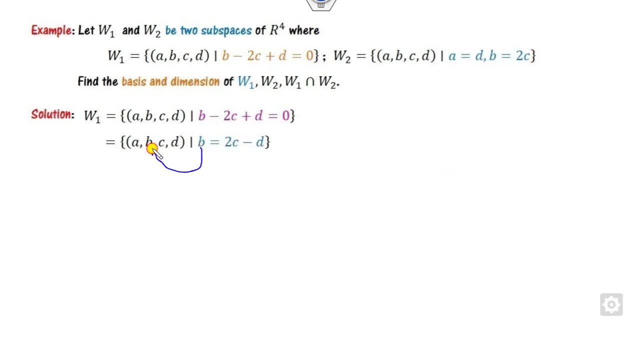 is quite easier. so i can write the value of b. substitute the value of the b. here you will get this. all the elements are written in terms of the c and d, so i can write a, c and d. so these three are my basis and the dimension is my 3. similarly, we can start from the w2, since a is equal to d. 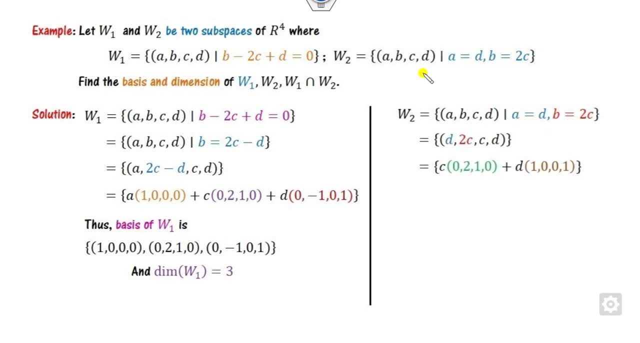 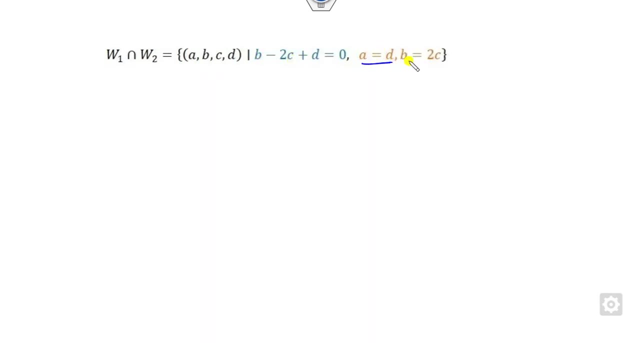 b is equal to c, so i can substitute the values at here. so you can see. these are the two are my basis. dimension is my 2. how you can find the intersections are there. so, since it is a, and, so i can write these two pairs simultaneously. now, since a is equal to d, b is equal to c, you can.